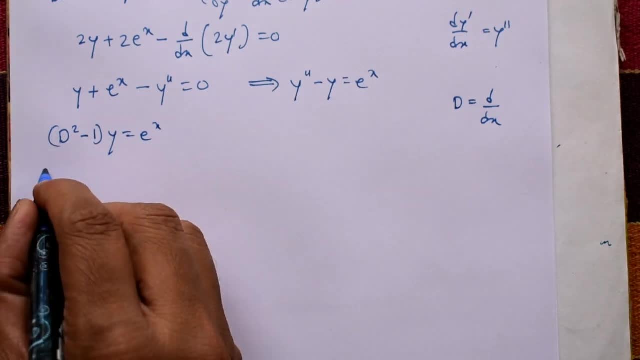 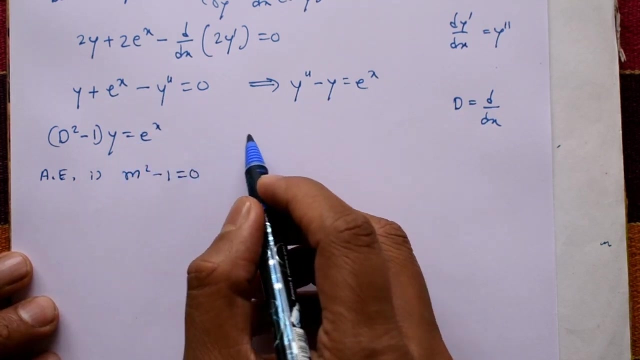 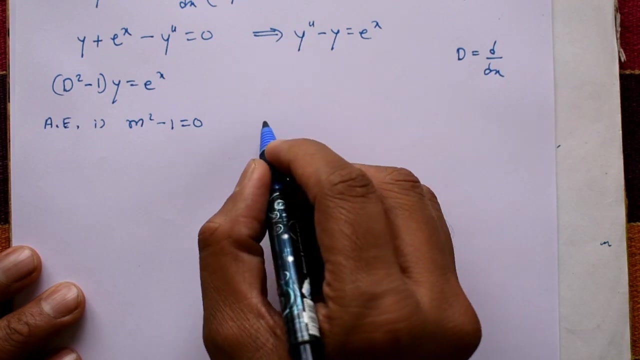 Okay, now find the general solution. First is a auxiliary equation: is m square minus 1 equal to 0.. Now general solution means finding the complementary function and particular integral. Now add complementary function plus particular integral. you get general solution. Now m square is equal to m, square minus 1 is equal, m square minus 1 equal to 0, or m is equal to plus or minus 1.. Now 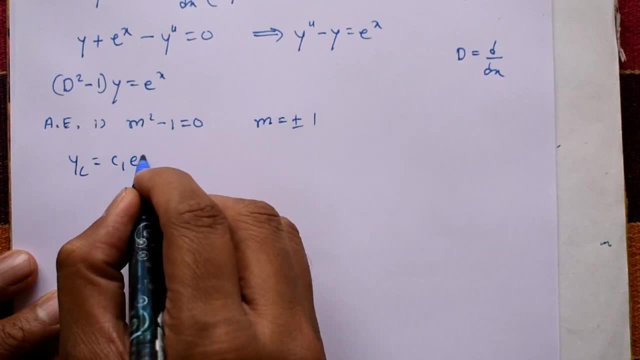 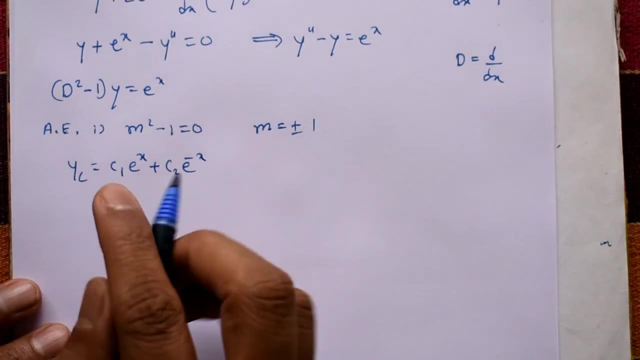 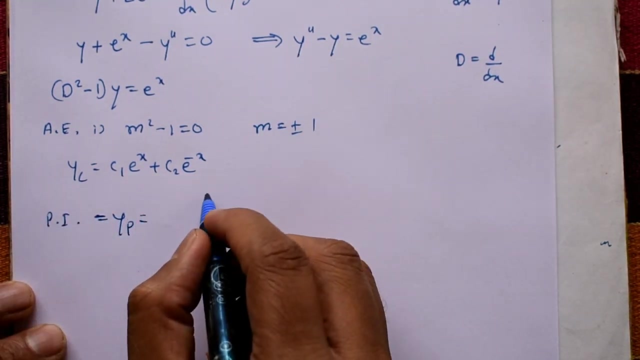 complementary function is roots different: c1 e raise to x plus c2 e raise to minus x. now comparative function is over. now go to the particular integral. okay now, particular integral is: are called yp. that is equal to e. raise to x, right hand side, whatever e raise to x upon f of d. this is f of d is. 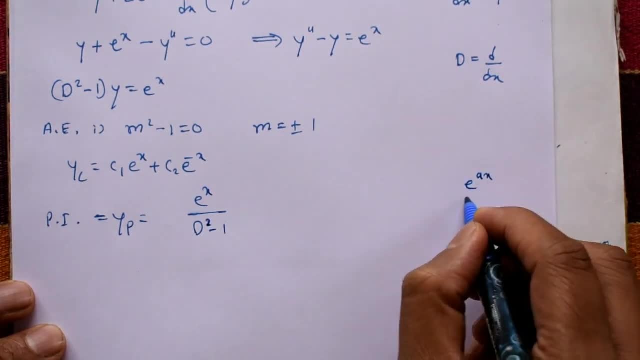 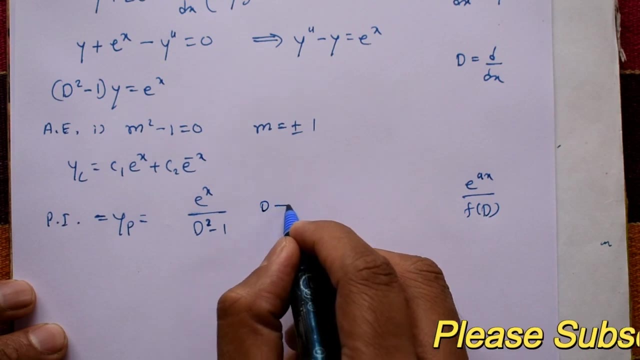 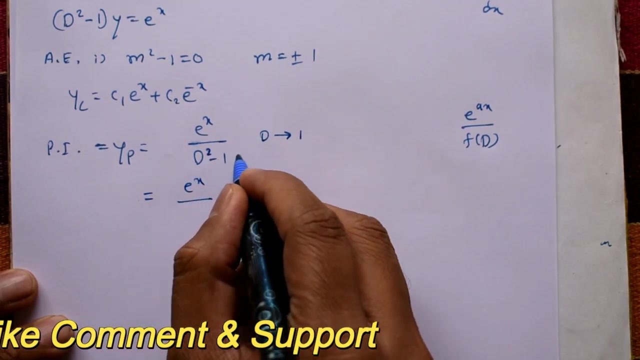 a d square minus 1 is a formula is like this: using this one, now in this case, you take d equal to a, a means 1. put d is equal to 1. now this is a e. raise to x: 1 minus 1, d is a 1. 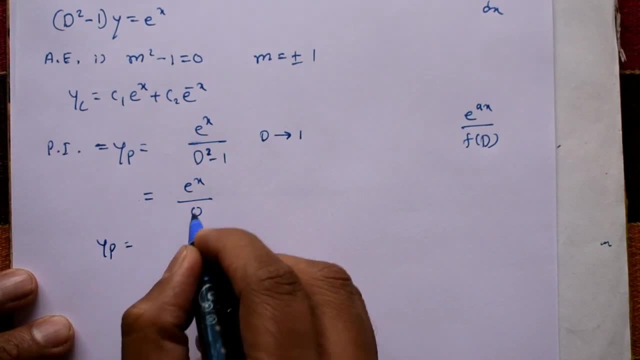 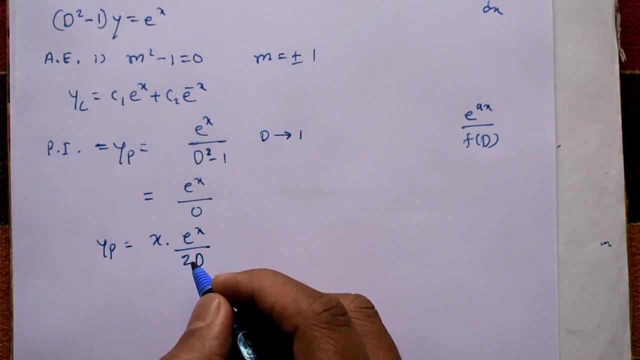 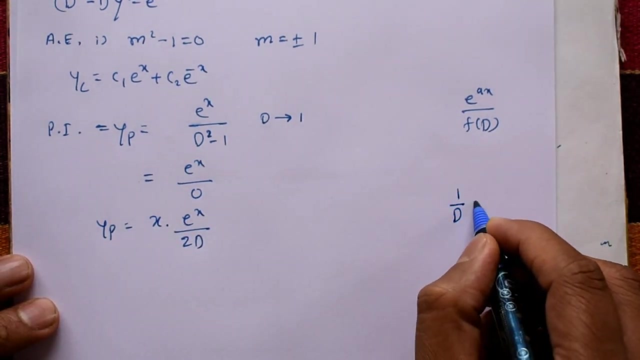 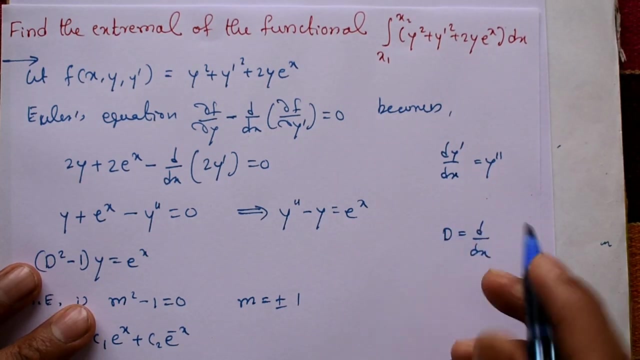 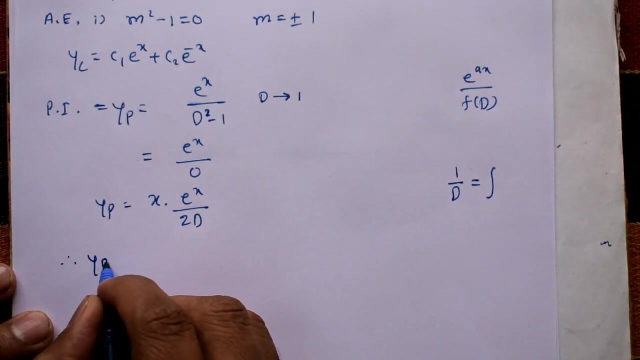 that is 0. okay, now that time. multiply by x and e, raise to x and differentiate this denominator, you get 2d. okay now, now d stand d by d x, but 1 by d is integration. inverse differential operater. now, this is a differential operator. d is a d by d x and 1 by d is a inverse cottm. 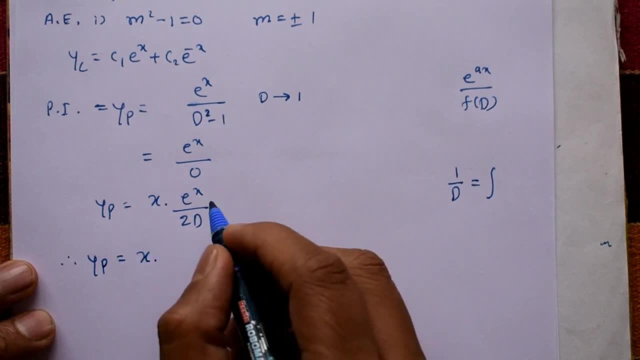 itez means integration. now, Thereforeparticular integral is x into integration of e raise to x. only integration of e raise to x is e raise to x, and two is about this. Sothis is the previous step, and then the next step is the first step can be followed. 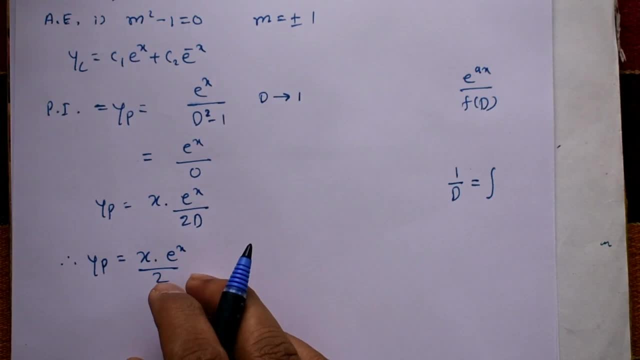 Sowe are doing now어�ere hubs the general principles of E raise to x space resolution. ei raised to x plus, e raise to x plus or has to be m? e raise to x plus is a constant as it is x into e raised to x by 2. this is yp. now general solution is: y is equal to. 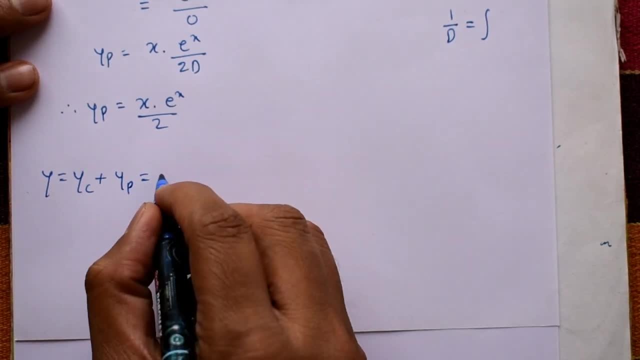 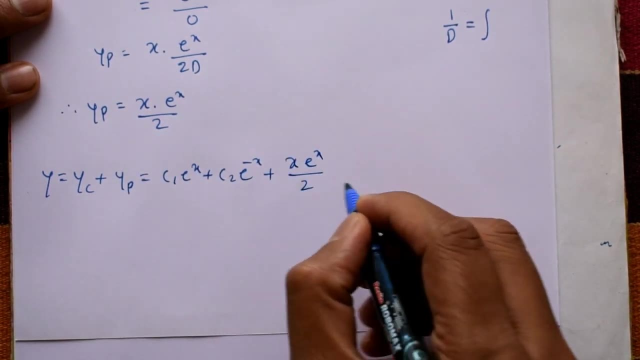 complementary function plus particular integral. now complementary function is c1 e raised to x plus c2 e raised to minus x plus particular integral is x into e raised to x by 2. now this is required general solution.